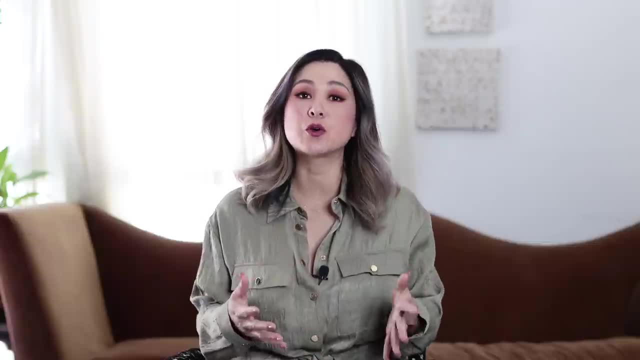 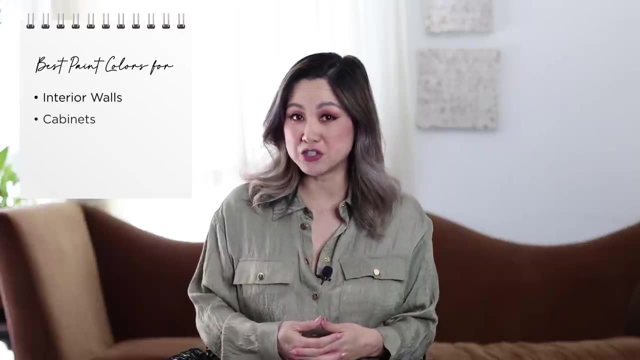 I'll be breaking down the colors that pair perfectly with natural red brick this video into four main sections. First, we're going to tackle the interiors. We're going to take a look at interior spaces that feature brick walls. Next we're moving on to cabinetry, and I'll 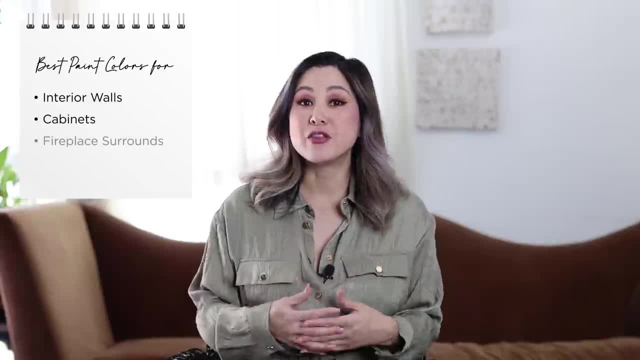 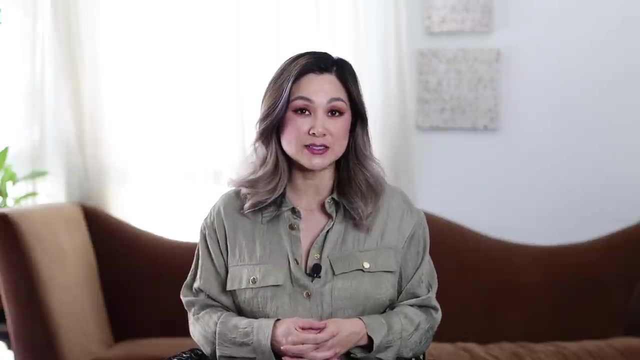 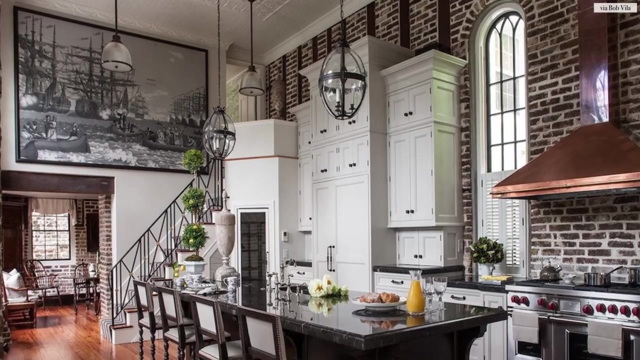 be sharing my favorite cabinet colors to pair with brick. Then we move on to those brick fireplaces and we will end with exterior brick facades. Let's talk about those interior spaces. Natural materials look best paired with the natural finish of raw, unfinished red brick From a stone fireplace to 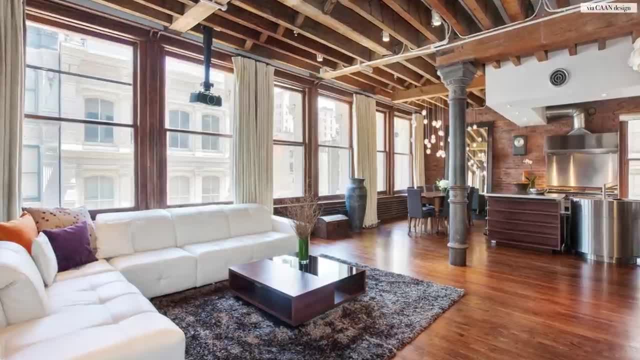 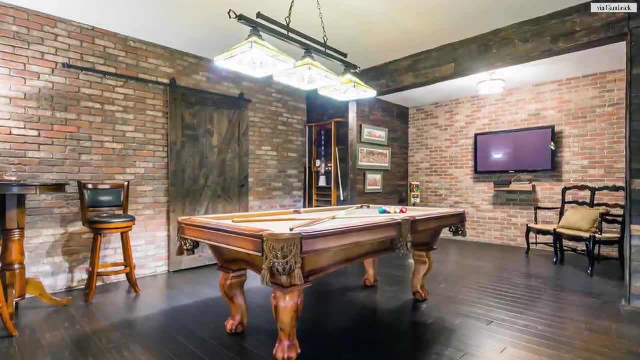 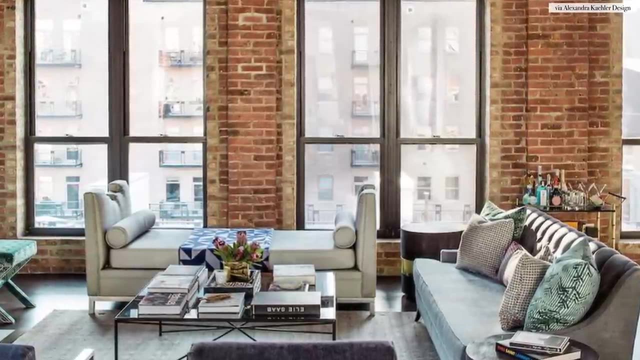 a copper hood. we're going to take a look at the interior spaces that feature brick walls: From distressed wood beam ceilings to reclaimed wood-paneled walls. look to colors found in nature to inspire the color of paint or stain on your walls. Red brick is such a bold statement in itself. so you're looking to move away from those red sunset. 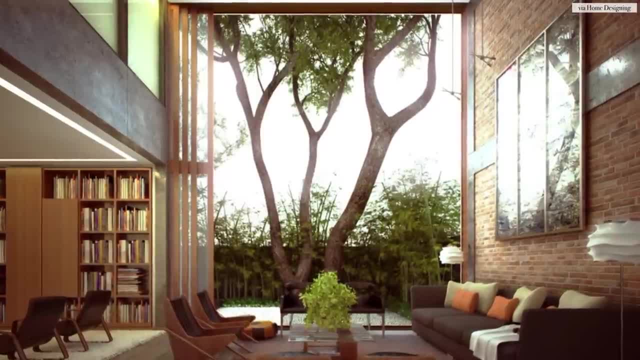 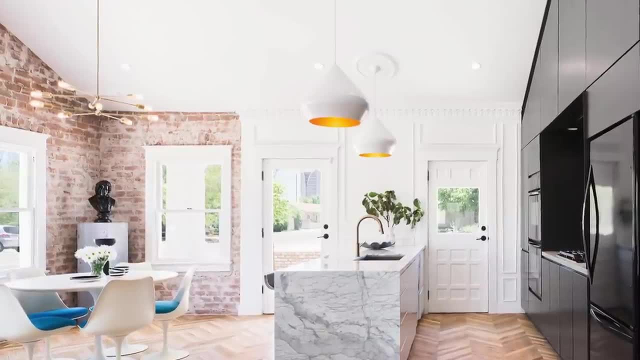 hues like golds and oranges into cooler tones to bring out the natural beauty of unfinished brick. With this in mind, you want to look for cooler whites, cool tints like blues, grays and greens and, of course, you want to look for a color that is a little bit more natural. 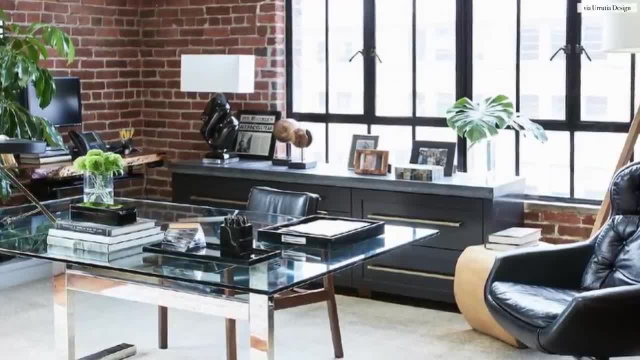 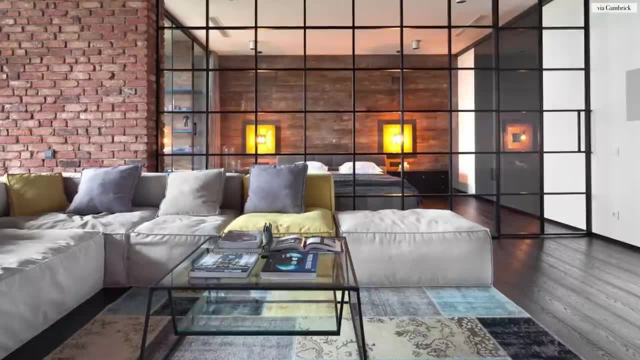 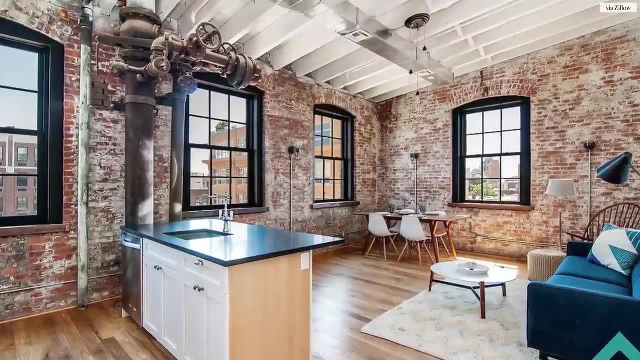 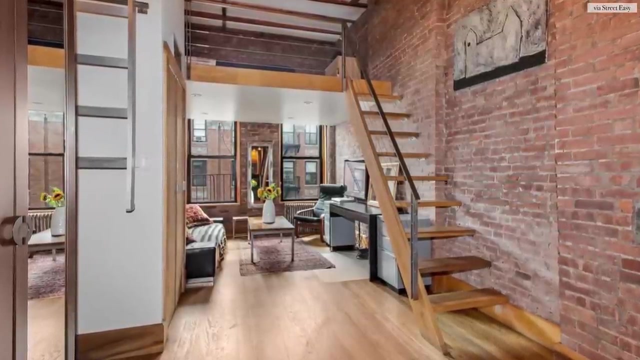 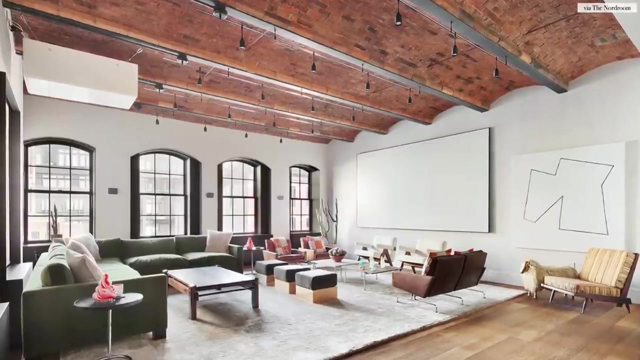 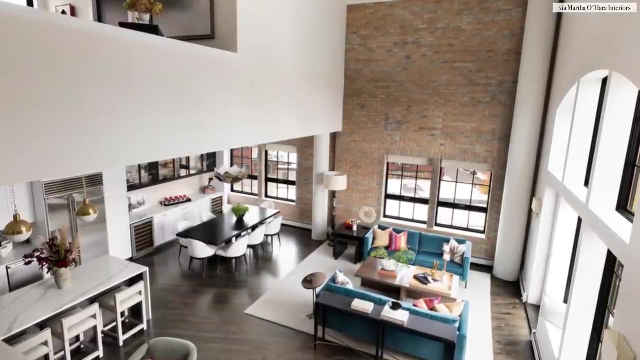 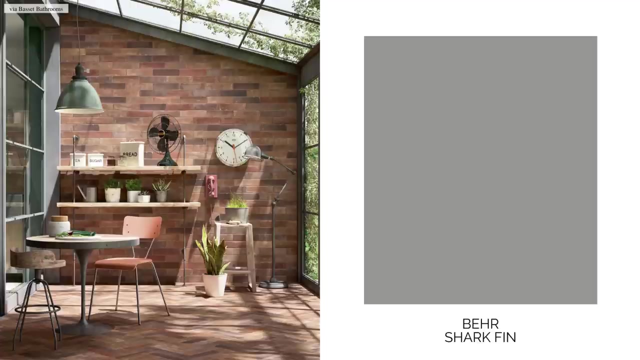 You know how I love to add black accents to modernize any interior space. I love how bear shark fin almost has a greenish undertone to the gray which looks beautiful against the natural landscape surroundings. I love how bear shark fin almost has a greenish undertone to the gray which looks beautiful against the natural landscape surroundings. 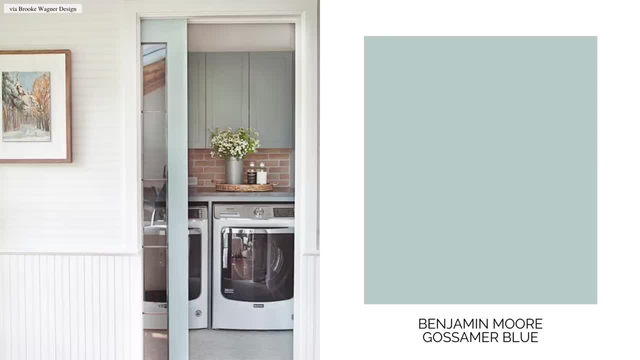 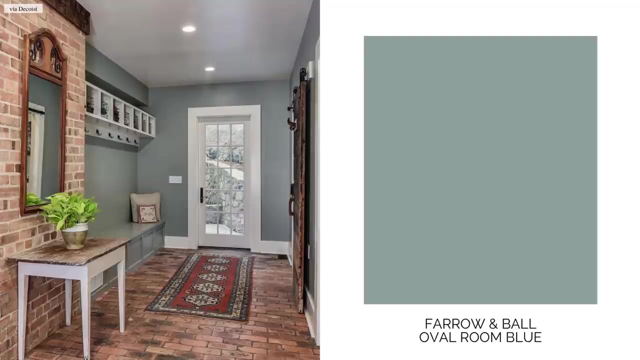 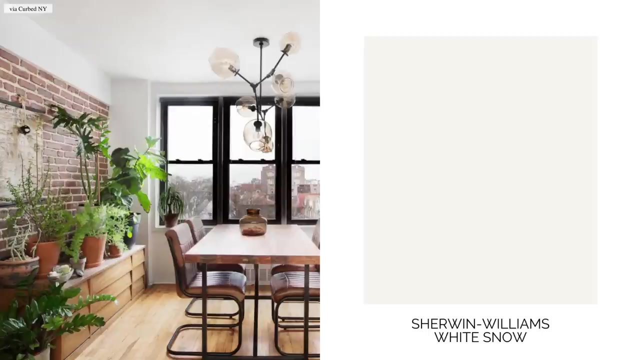 The light blue tint in Benjamin Moore's Gossamer Blue really brightens this laundry space and makes it look so unique for this modern farmhouse vibe. Sherwin-Williams White Snow is a really beautiful, pure, cool white that looks awesome against the indoor junglo of this industrial loft. 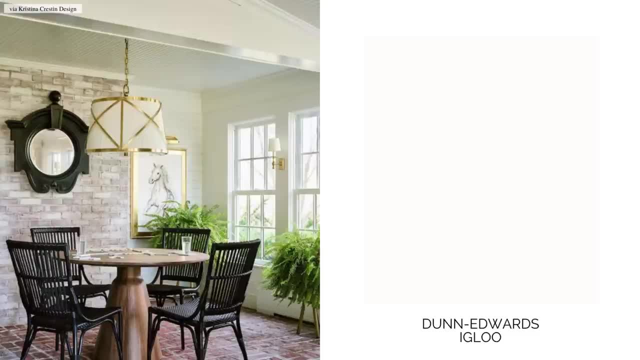 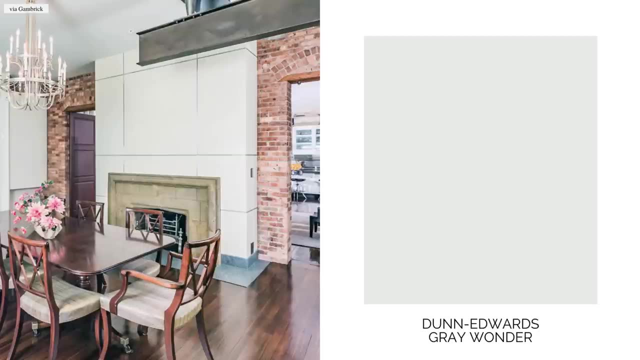 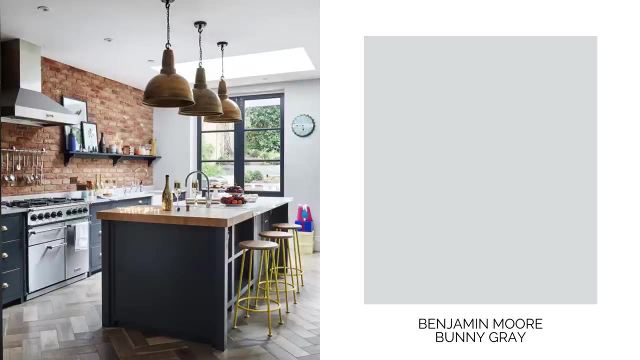 that looks awesome against the indoor junglo of this industrial loft. For transitional spaces like this dining room, Dunn-Edwards Gray Wonder is such a cool twist on a modern white. Dunn-Edwards Gray Wonder is such a cool twist on a modern white. 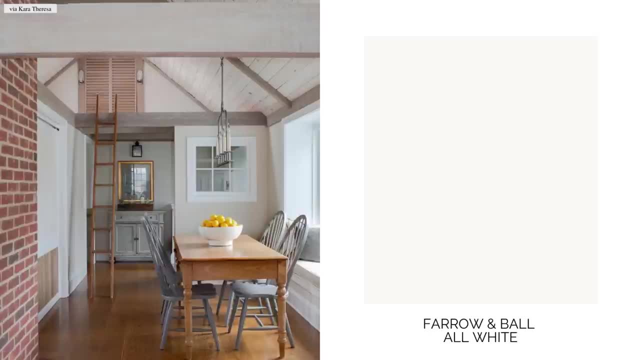 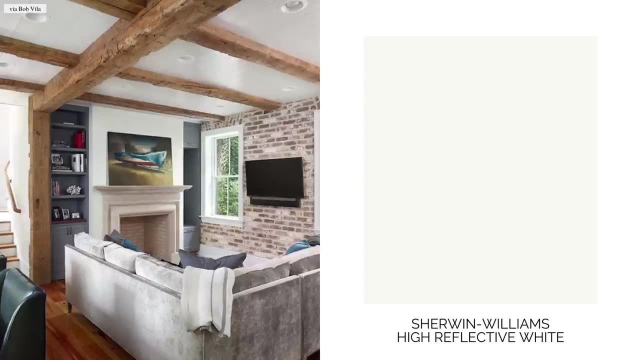 You can't ever go wrong with Farrow & Balls All White. I love how it warms up this cottage-style dining space. I love how it warms up this cottage-style dining space. I love how it warms up this cottage-style dining space. 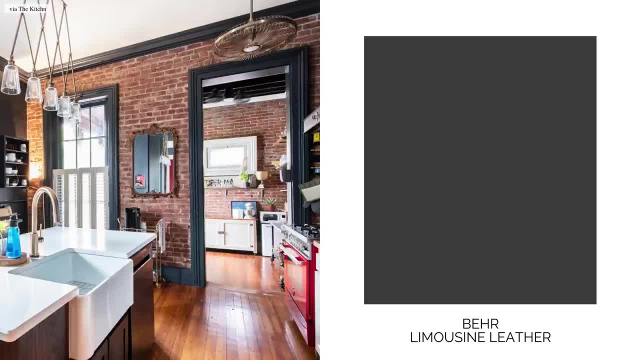 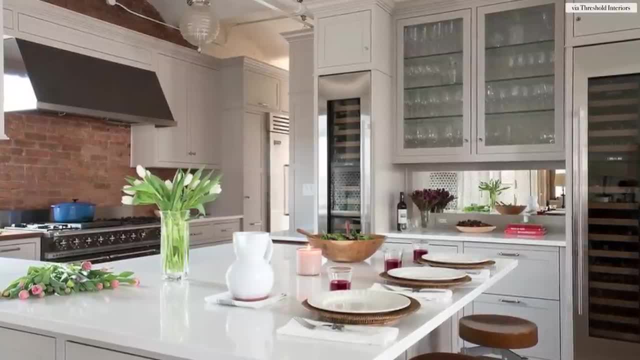 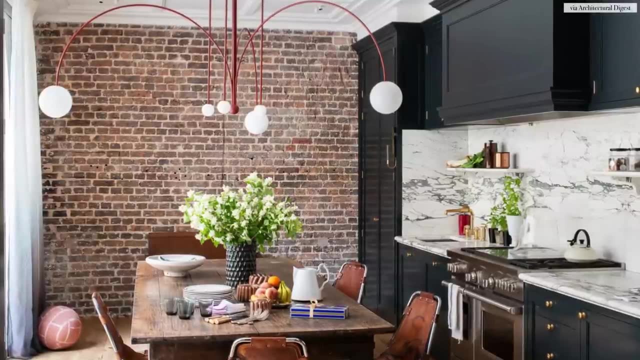 in this case, you might already have your color picked out, but need to find something equally as special as the brick for your cabinets. you could go bold with highly pigmented, dark, moody hues in the blue, gray, green and black family. a designer's tip when going dark and bold with 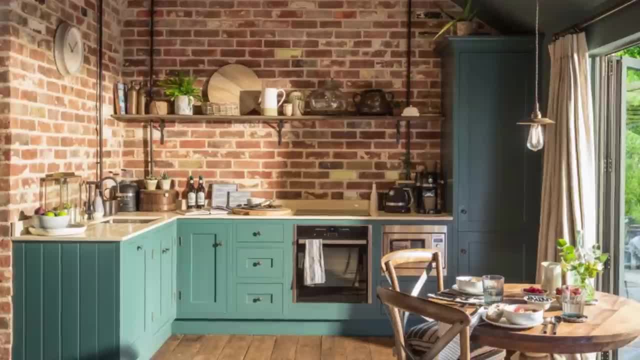 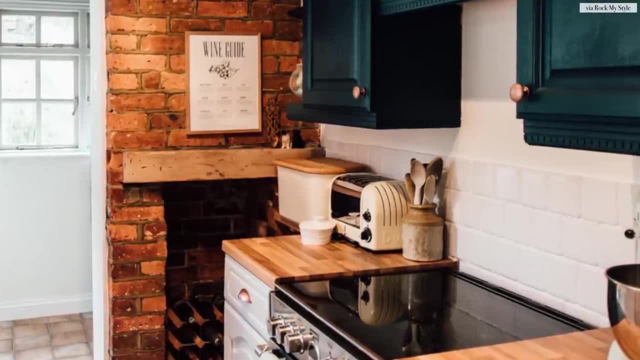 cabinetry is to make sure there's high contrast in the form of a white countertop or light backsplash. doing so will allow the space to feel light and bright instead of too dark and too cold. by definition, brick has the capacity to warm up a space simply by the color alone, but strategic. 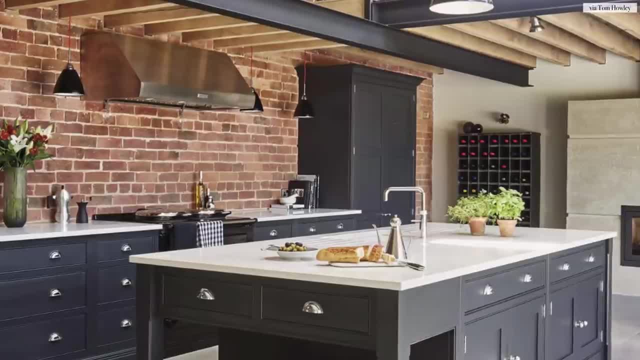 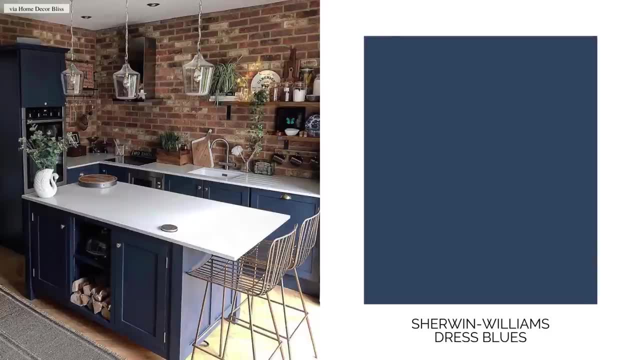 design moves like bringing in more contrasting paint pairings can help modernize it and make it feel current yet timeless. if you're looking for a bit of color to amp up the kitchen, how about sherwin-williams dress blues? this dark navy lends a nautical twist to an otherwise very contemporary. 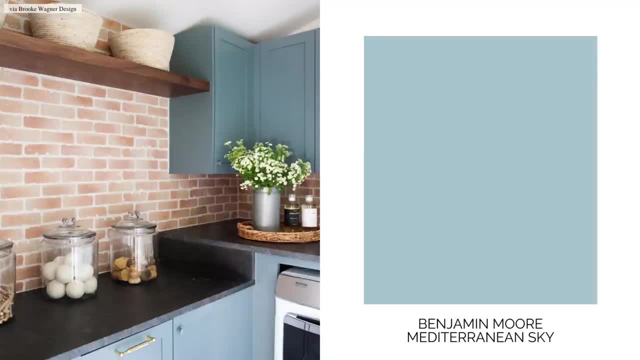 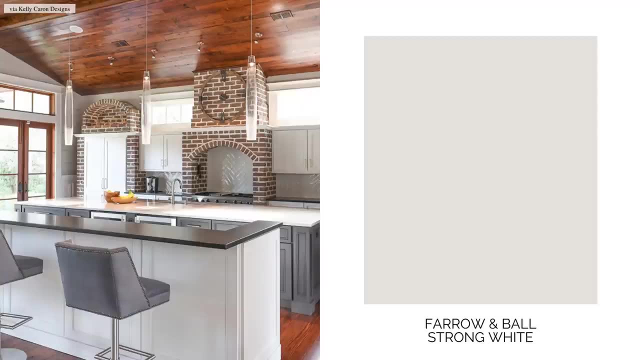 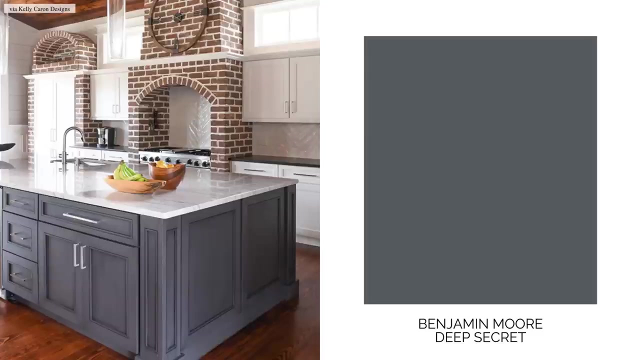 kitchen. here are two takes on the very same kitchen: ferro and balls. a strong white color painted on the cabinets give this contemporary space a very classic twist. how about choosing a contrasting island in benjamin moore's deep secret? this is a great way to break up a really huge kitchen. 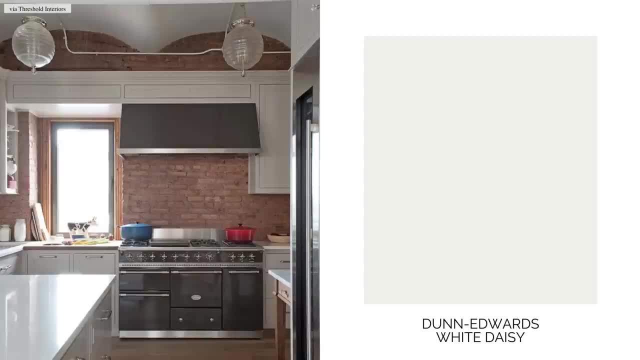 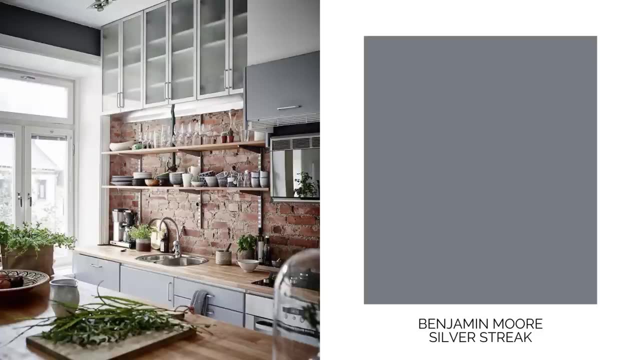 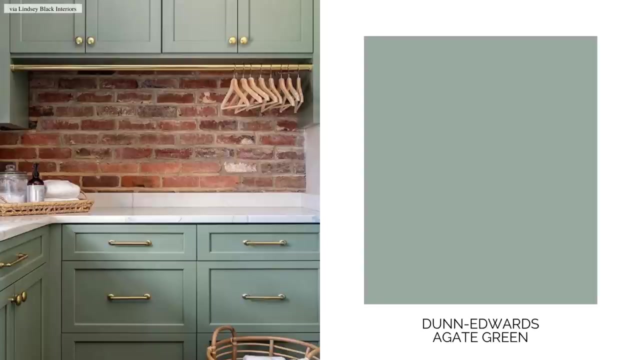 and give it some modern appeal. i am living for dunn edwards agate green in this laundry space. on the color wheel, green is found opposite from red. green is a color of the year and for good reason. it feels so calming and serene in this busy space. if you're looking to make a bold statement with bold color, how about sherwin-williams? 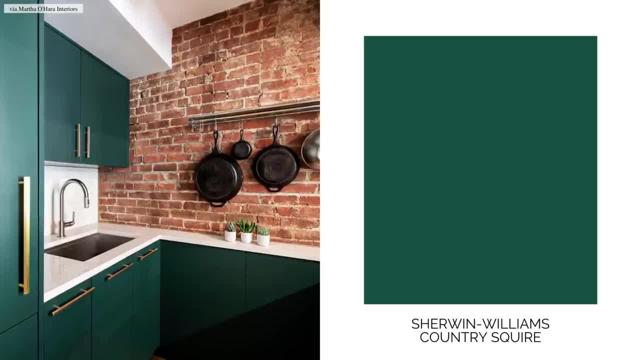 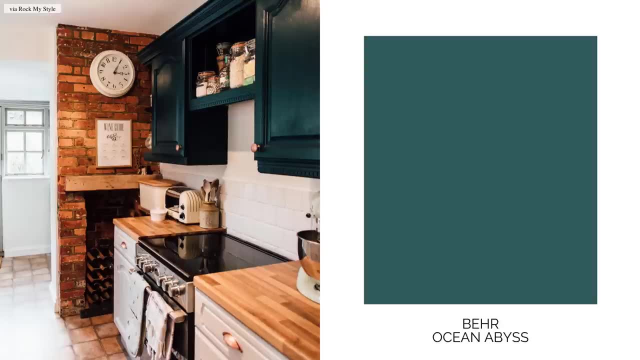 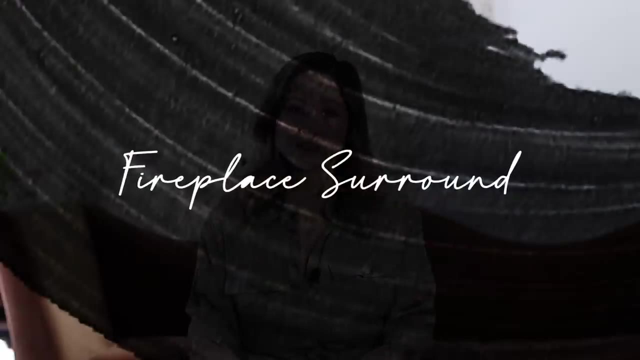 country squire. this jewel-toned green makes this small corner kitchen look so sophisticated and chic. the most common place in your home that you would find raw natural brick is on the fireplace. you might be dealing with just a simple hearth surround, or your condition could be a bit more challenging. 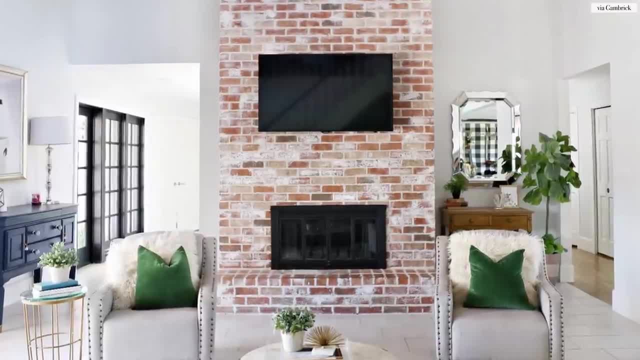 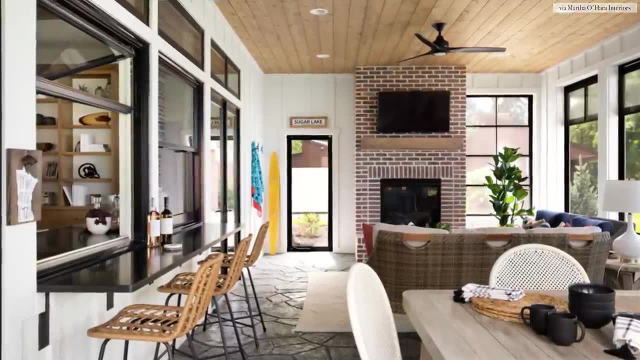 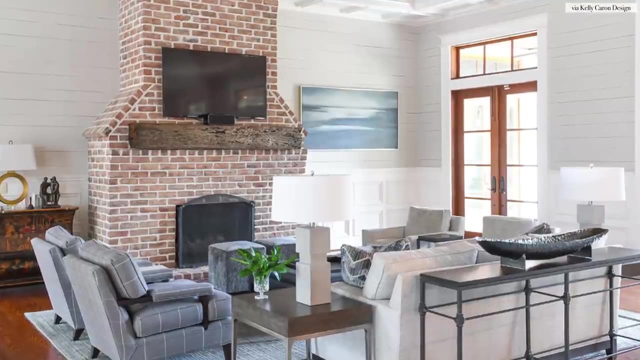 with a floor-to-ceiling natural brick elevation. whether you want to play up the feature or tone it down, make that design decision early on to help you select the perfect hue for your space. even though this portion of the wall has been lime washed, i love the way benjamin moore's 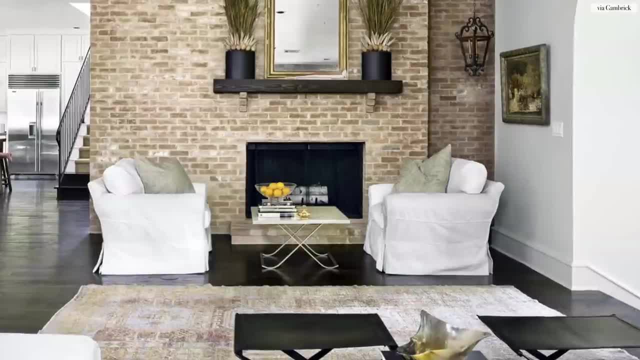 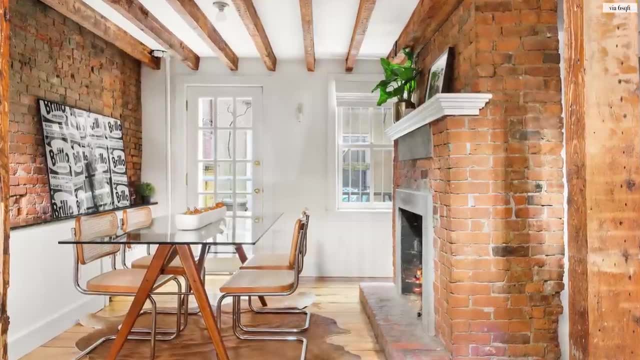 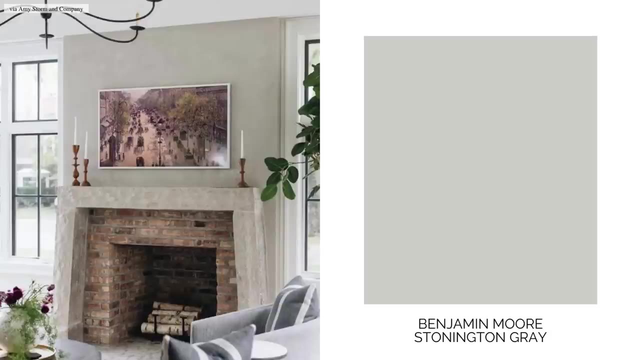 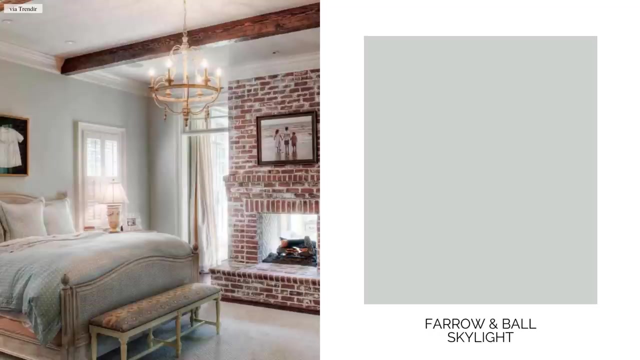 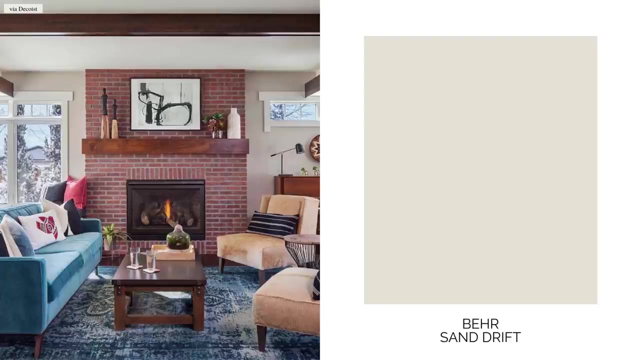 stonington grey really plays down the color of the brick. it's almost akin to pulling the grout color to inspire your design. you can't go wrong with� outer hiện with a color that mimics natural stone. Bear's Sand Drift is a really beautiful light grayish. 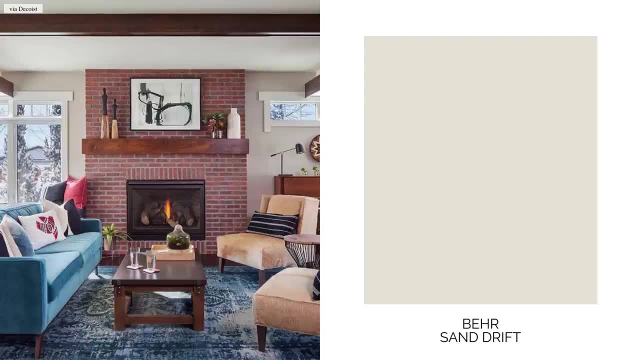 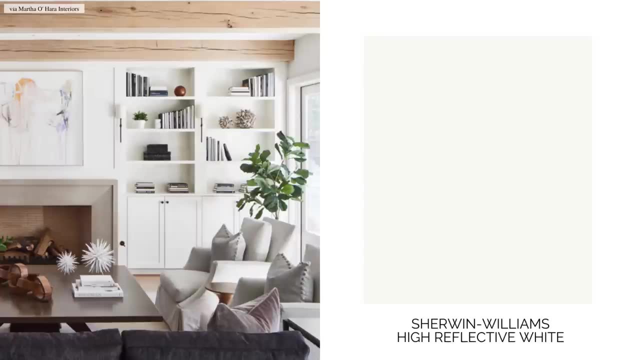 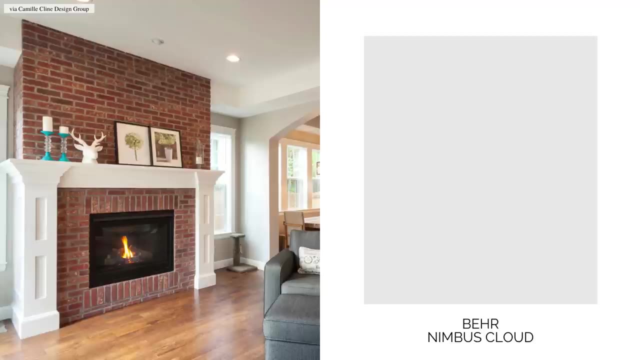 which is a combination of gray and beige. I love how this cool color tones down the redness found on the brick facade and the wood mantle. I love how this color tones down the redness found on the brick facade and the wood mantle. I love how this color tones down the redness. 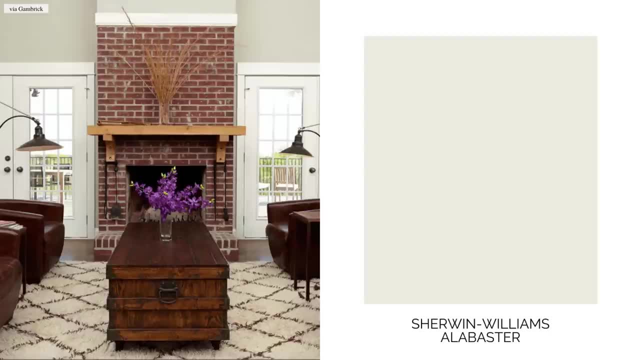 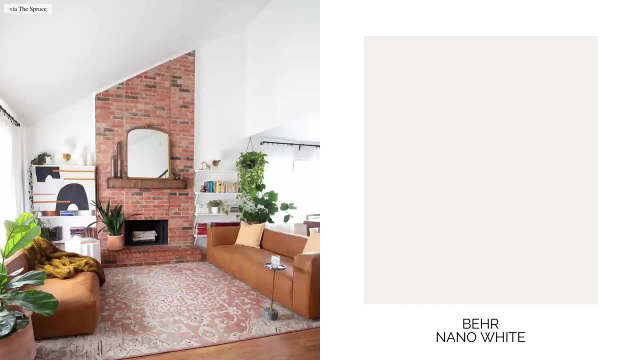 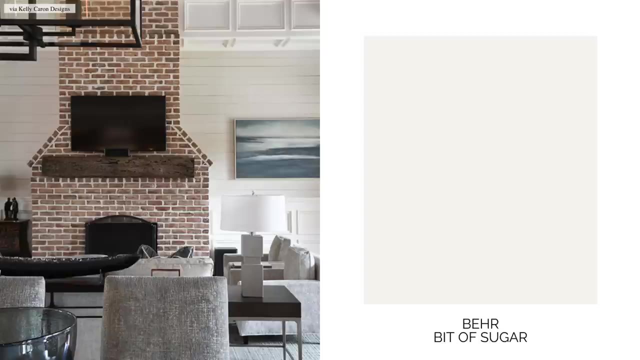 found on the brick facade and the wood mantle. Sherwin-Williams Alabaster is a little bit more warm, so if you have a lot more daylight in the space you could also use this color against a full brick elevation. You know I love those dark. 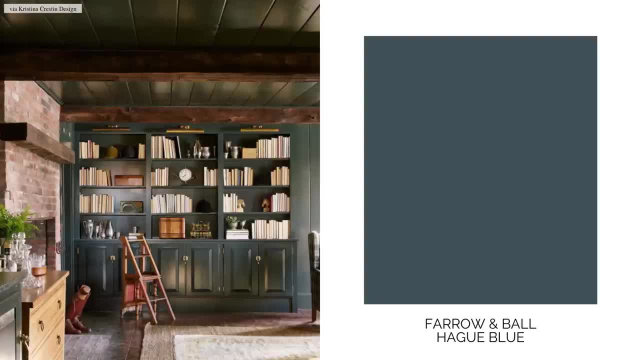 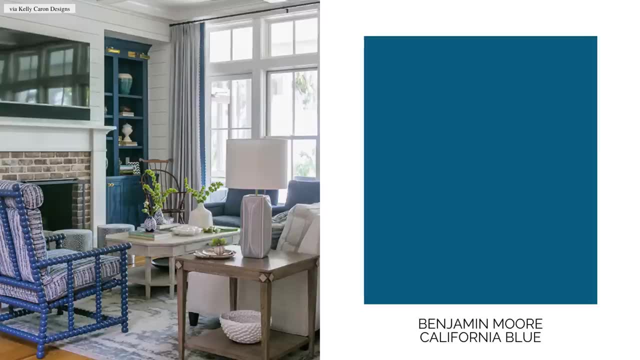 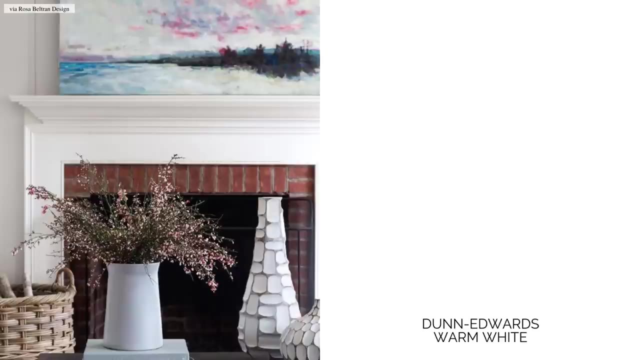 moody hues, so Farrell and Ball's Hague Blue is such a beautiful contrast against natural brick, especially on bookshelves or a library. Looking for the perfect white, Look no further than Dunn-Edwards Warm White. I've used this color for a ton of clients. 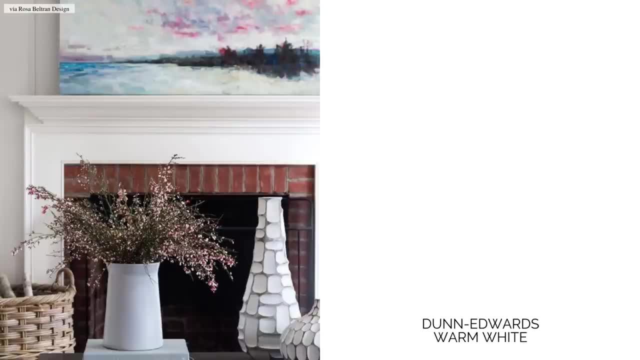 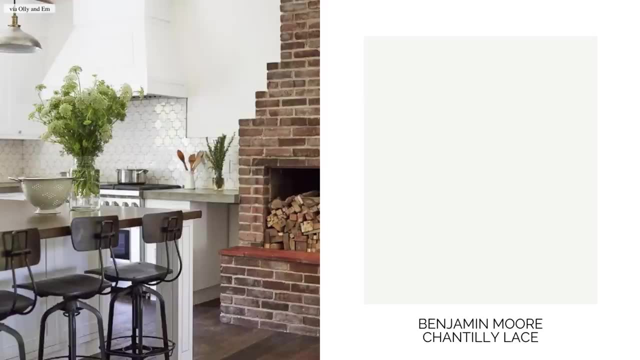 in so many different types of interior styles, from modern to transitional to classic, contemporary and even coastal. Every room looks great in warm white. Every room looks great in summer. Every room looks great in winter. Every room looks great in spring. 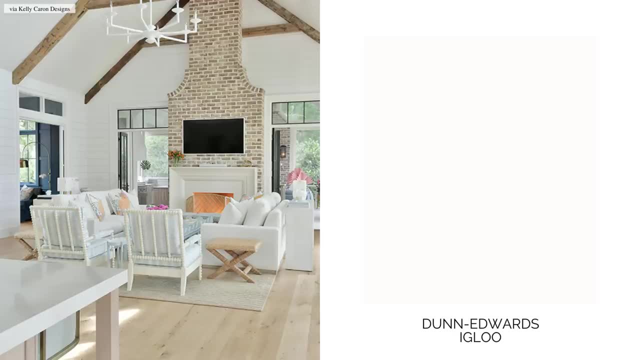 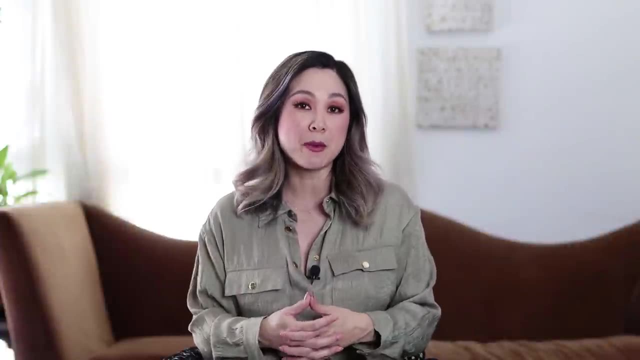 Every room looks great in fall. Every room looks great in winter. Every room looks great in spring. Every room looks great in winter. The entire concept behind this video is for all of the viewers who wrote in, If you recall, from my best exterior paint colors. 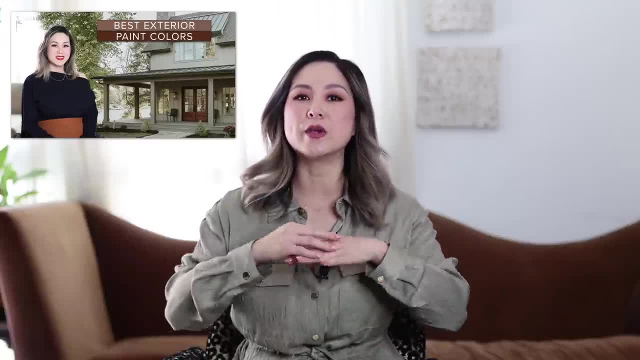 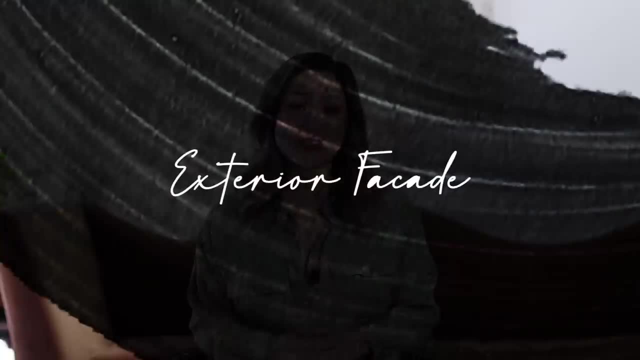 to help boost curb appeal. so many of you wrote in and said: we have brick on our facade and we are not painting it, we're not distressing it, we're not lime washing it, we're keeping it in its current state. 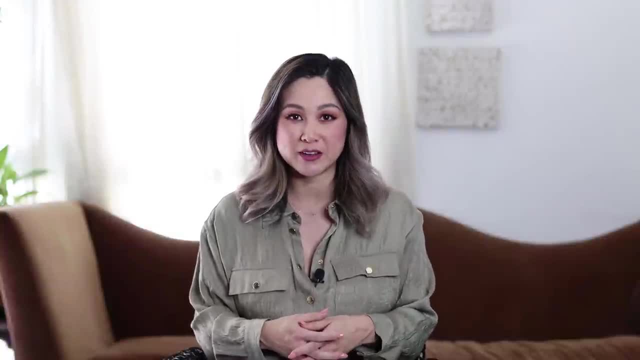 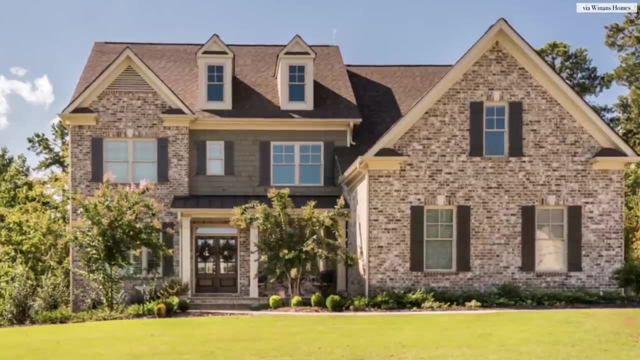 What are the best exterior paint colors to pair with natural brick? My team and I spent hours upon hours searching for inspirational exterior home colors, but so many of you wrote in stating that natural brick was the biggest challenge that you face when looking for the perfect paint color. 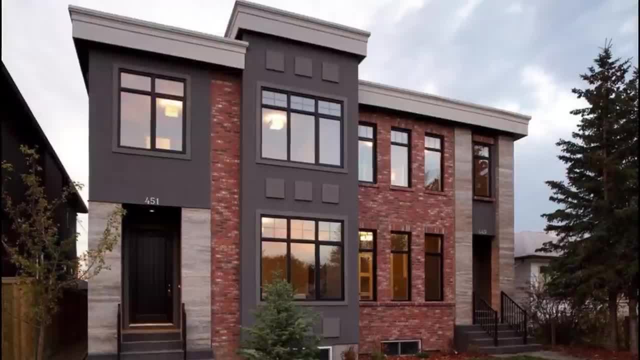 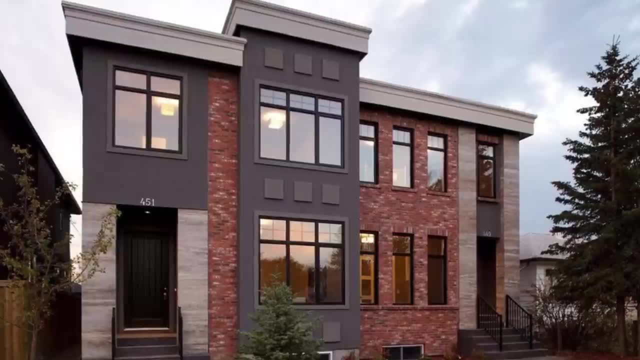 for body trim details and doors. I hope these next slides will help you lock down a color that you're absolutely obsessed with to bring out the true color of your existing brick facade. Cottage-style homes with traditional white trim always need a bit of contrast. 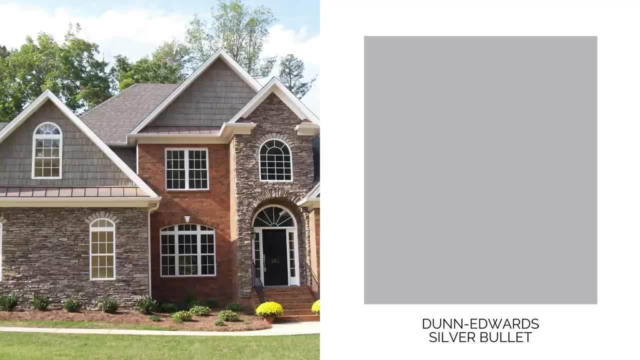 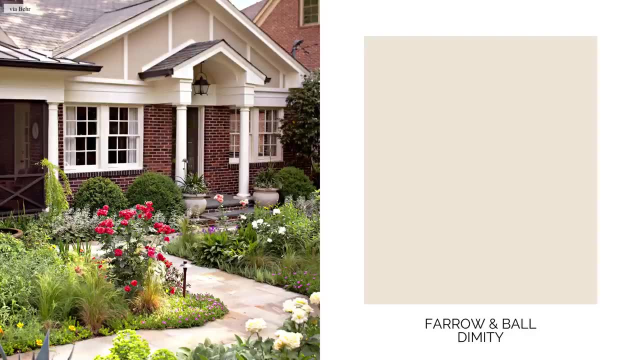 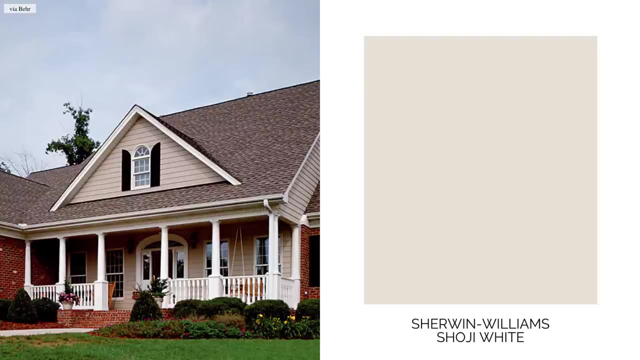 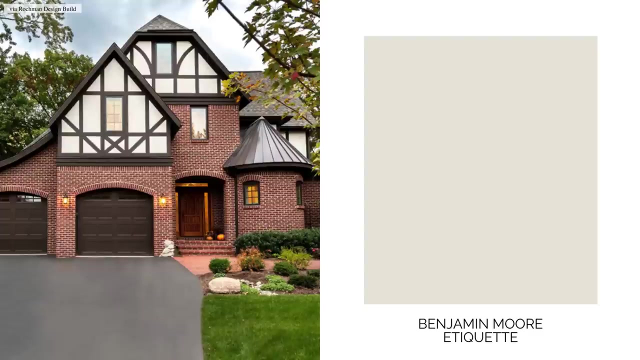 Whether you're going light, like Benjamin Moore's Bruton White, or dark like Dunn-Edwards Silver Bullet, think about your natural surroundings and consider how much sun or shade your home gets. There are so many stunning dark and inky hues. 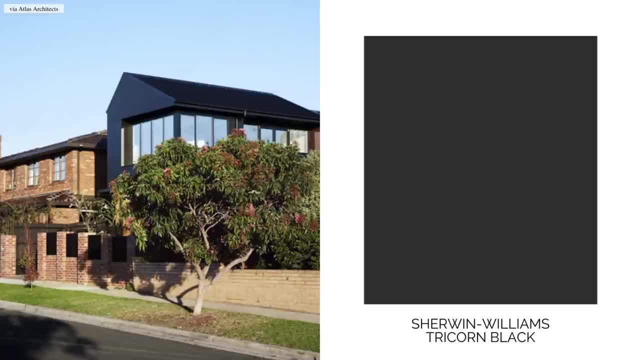 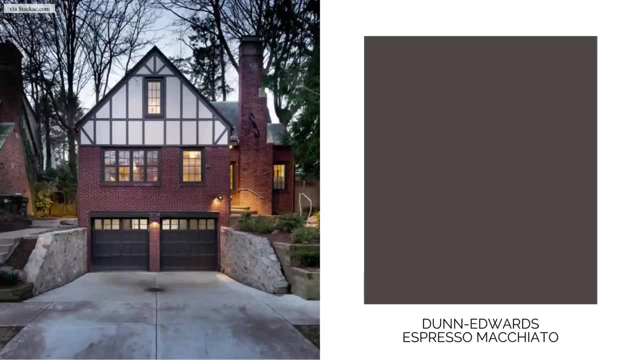 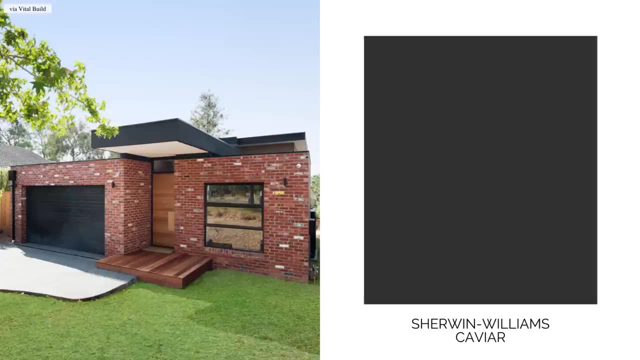 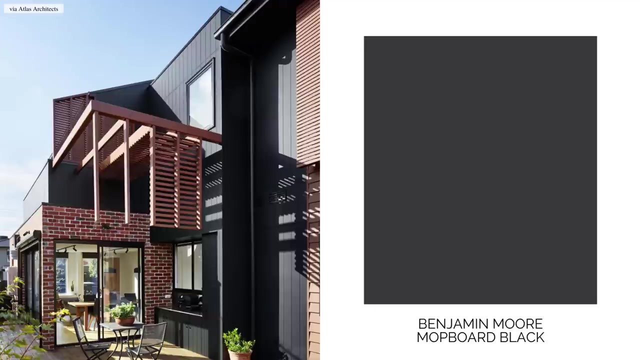 that work beautifully with natural brick. Look to your particular house style and see which fits best for you. There are so many stunning dark and inky hues that work beautifully with natural brick. Look to your particular house and see which one looks the best for you. 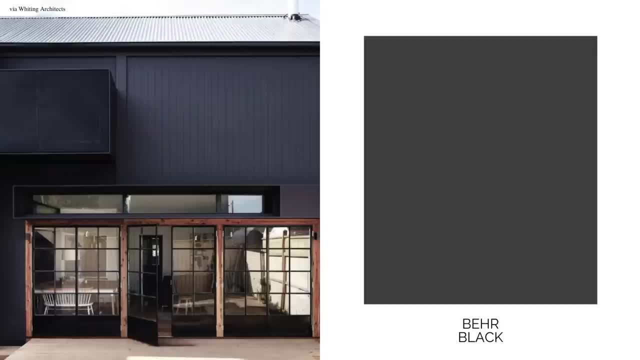 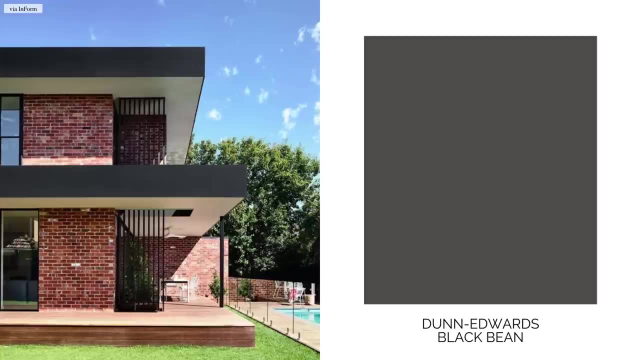 Make sure your home is perfect. When you live in a natural brick house, try to sift and scale your building and design a little bit more to make the home look like a natural gold, And if it looks like a natural brick, that's right. it's not. 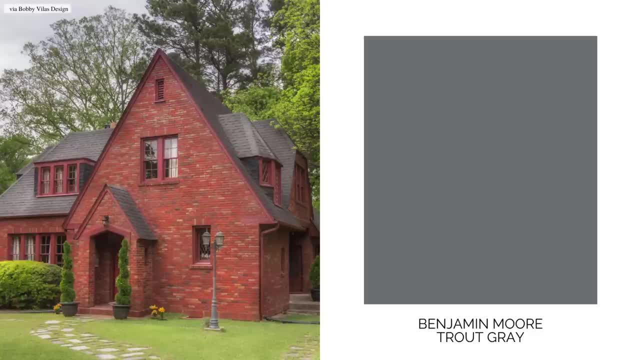 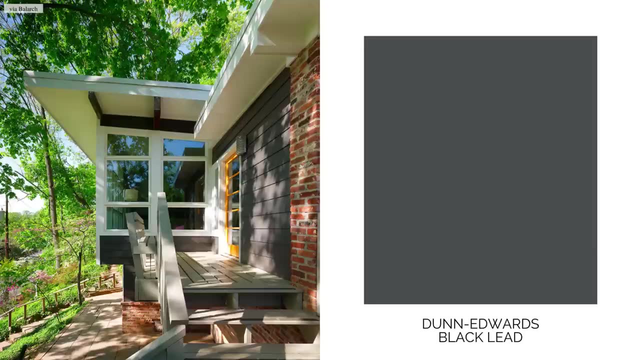 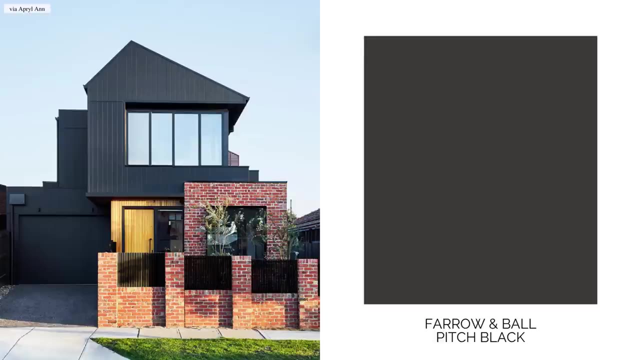 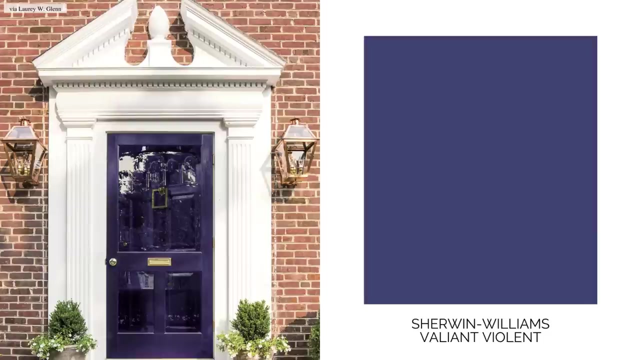 and it's much easier to master. Every time we paint, the challenge is to figure out how to make it look natural. So that's really the challenge right now. So I'm just going to stop there. If you're not ready, to go bold with pigmented wall color, how about a bold statement door? 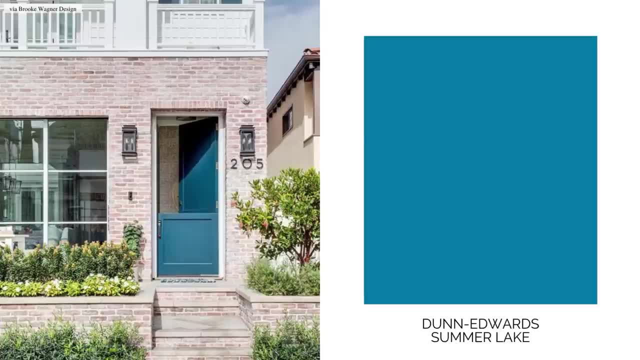 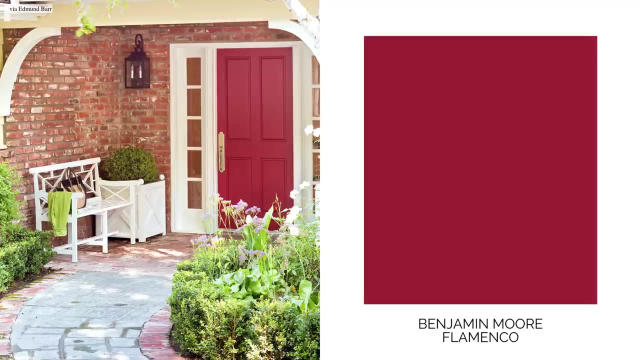 for size. I love Dunn-Edwards Summer Lake. Blue just looks too cool against this natural brick facade. Dunn-Edwards Summer Lake just transports me to the 4th of July celebration. A red door on a home is like red lipstick on an outfit: It definitely makes a statement and it's all about. 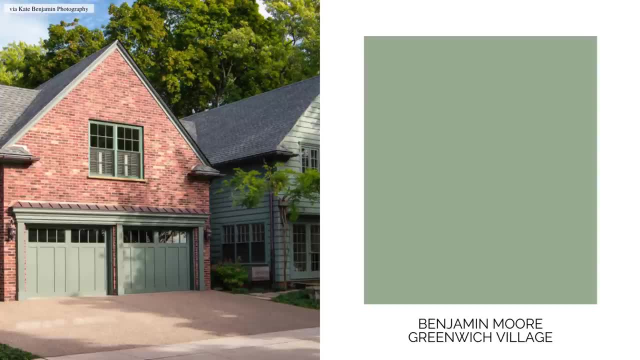 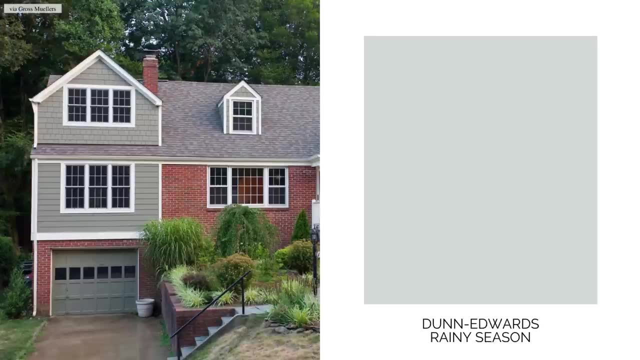 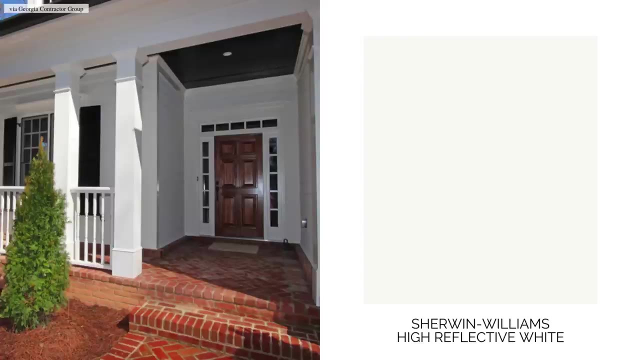 the hue. If you're looking to tone down natural red brick, think about paint colors with a tint of complementary green in it. Here are my favorite: neutral whites and off-whites to bring out the natural beauty of the brick and allow everything else to play a supporting role. 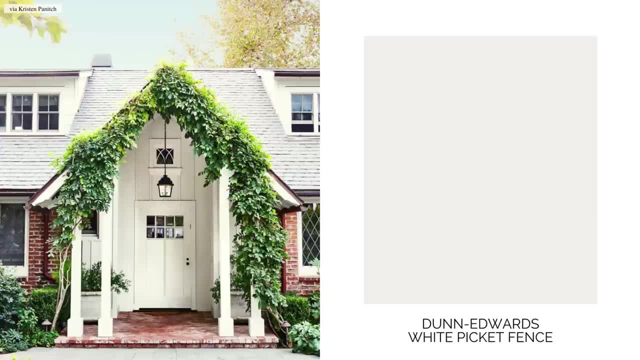 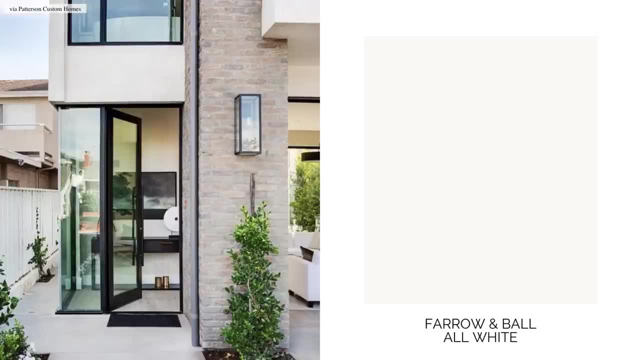 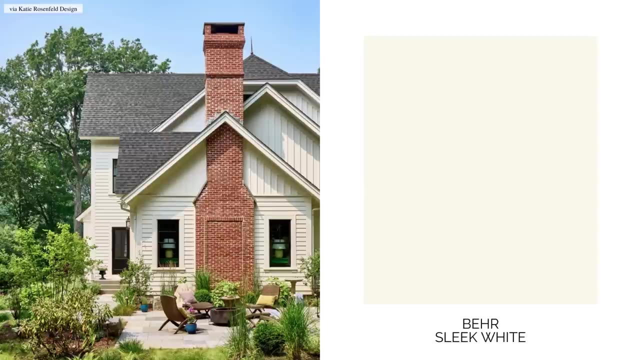 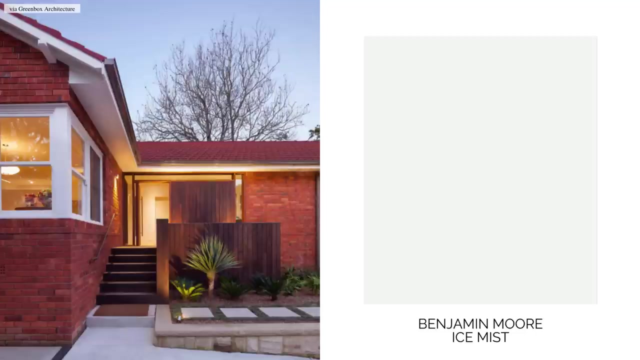 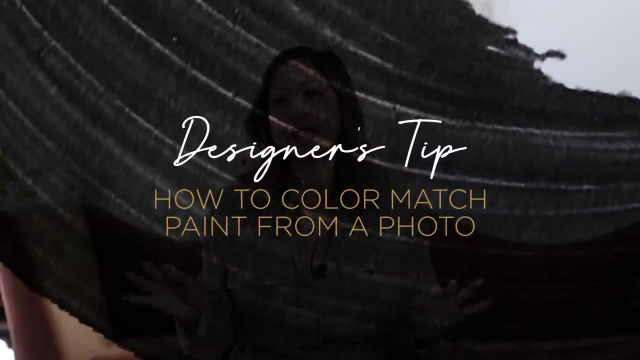 And finally, I want to leave you all with a designer's tip: Remember that you can't always be a designer. You can't always be a designer. You can't always be a color. match virtually any single color you'd like to any paint manufacturer, simply by using: 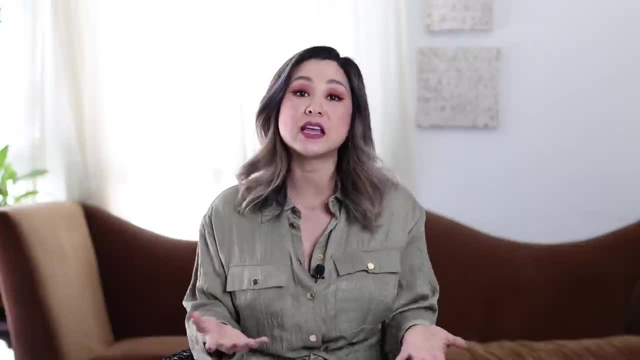 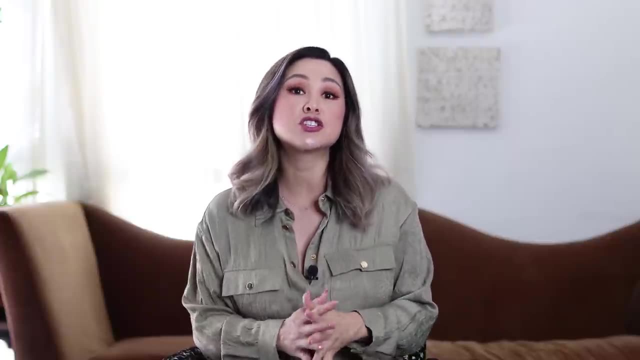 their application online. In this case, you can take a photo or you can save an image that you found online and you'll upload it onto the paint vendor's website and you can find a true color match. Let's use Sherwin-Williams as our example today. I want you to follow along this exercise. 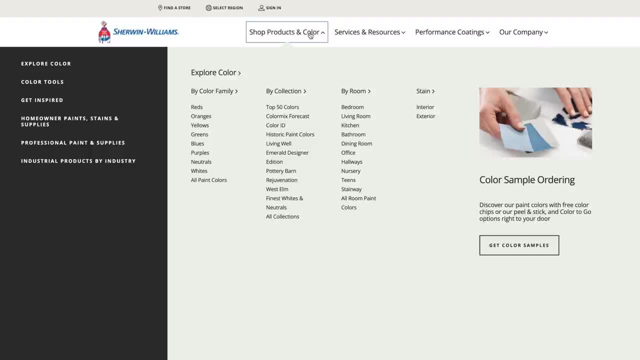 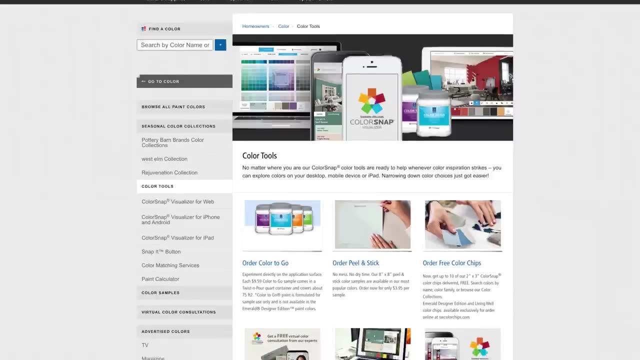 Try it for yourself on your laptop or the Sherwin-Williams smartphone app and see if you can find the right match for you. Find color tools in the left-hand menu. You'll scroll down until you see the ColorSnap Visualizer for web option. 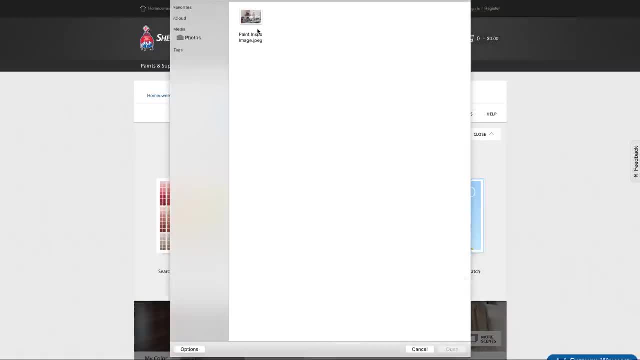 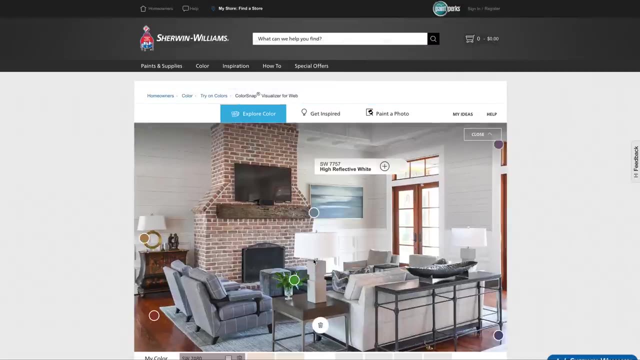 Explore color, Then match a photo From here. you can upload an image that you have saved onto your computer or photo gallery. if you're using your phone, The ColorSnap Visualizer will automatically find paint colors for you based on key details in that photo. If you want to match a color on the 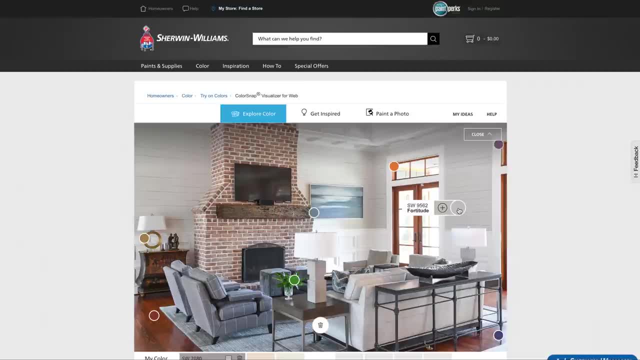 walls, move the cursor to that portion of the wall. As a default, the Visualizer will also match a paint color to the trim of the windows, the color of the wall and the color of the wall. You can also change the color of the rug, even the green on your indoor plant. This is a great way to not only 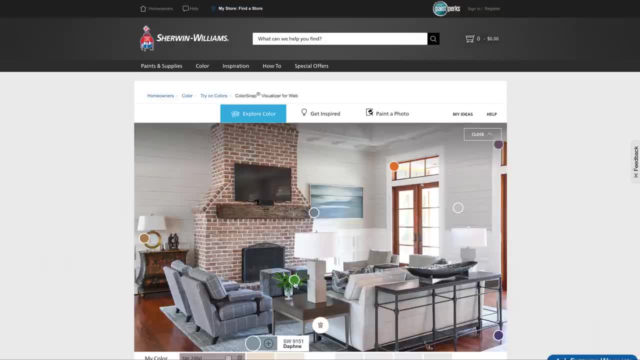 find a wall color from the photo, but accent colors. if you want to paint a ceiling or create a cohesive color palette for the room, to pull in accessories and artwork, You can move the cursor to a portion of the brick, even pull a particular blue from the artwork on the walls, Of course, 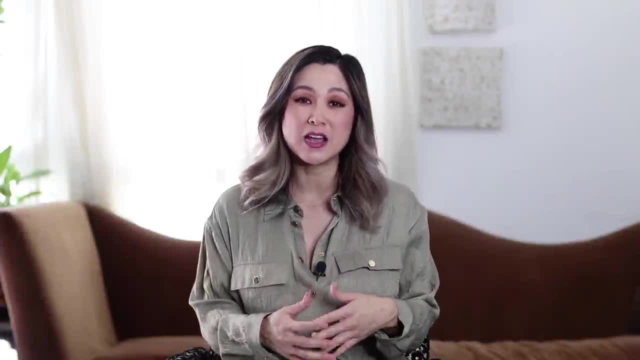 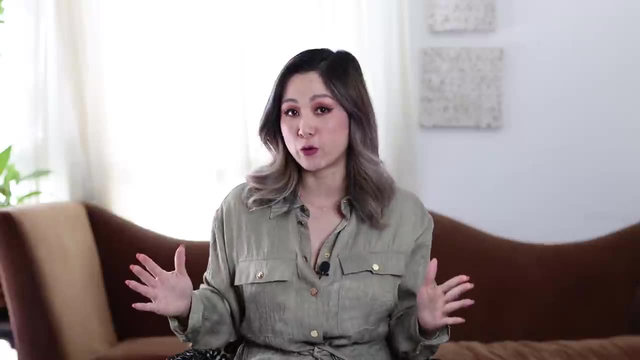 this Color Visualizer isn't always 100% accurate, so my advice is to always get samples and bring them home. paint them on the walls. make sure you paint 4x4 swatches like 4 feet by 4 feet. 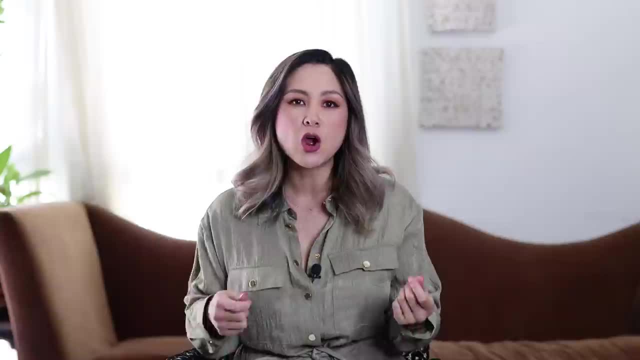 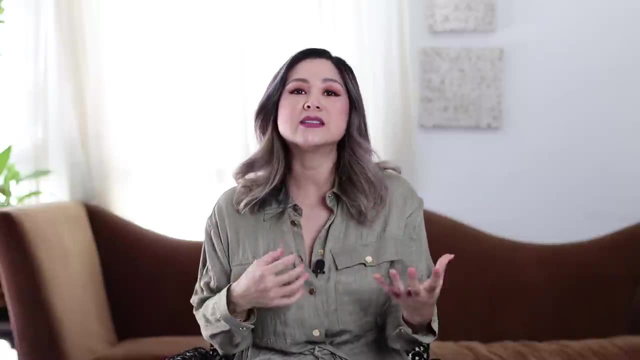 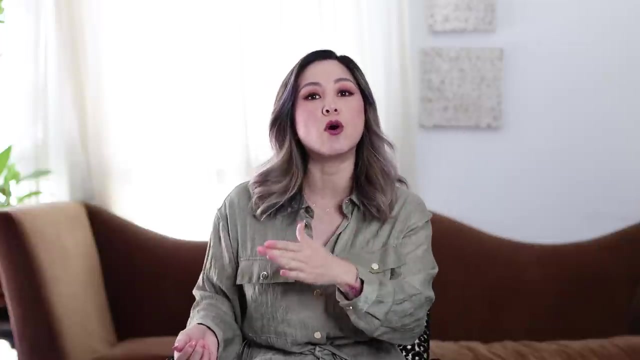 or large swatches on a prime piece of cardboard or some heavy cardstock. That way you can imagine in your space. you can pull these cardstocks around from wall to wall and see how the lighting changes the color of the hue. You could also do as the pros do, which is paint that swatch on every single.